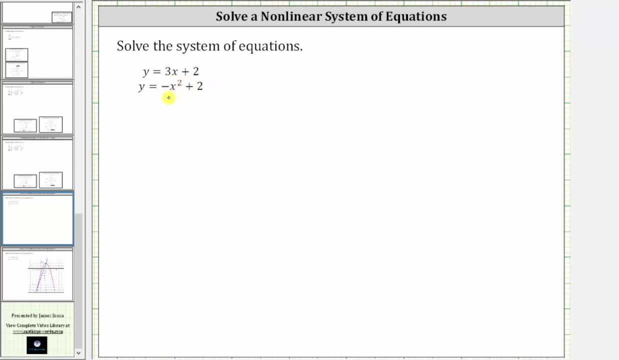 Because both equations are solved for y. we will solve this system using the method of substitution, where, because y is equal to three x plus two, we can substitute three x plus two for y in the second equation. By doing this, we will then have an equation. 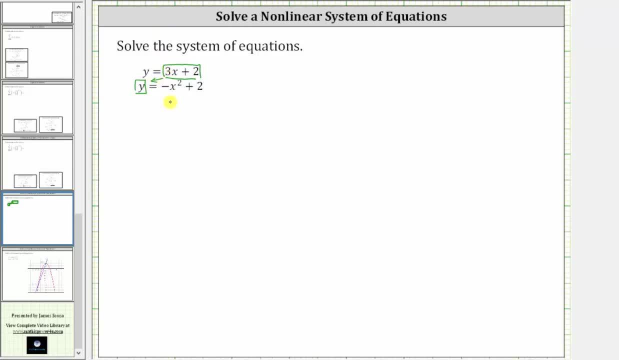 in one variable that we can then solve for x, But then we'll have to come back and determine the corresponding y values. Remember, each solution is an ordered pair in the form of x comma y. So, performing the substitution, we have the equation three x plus two. 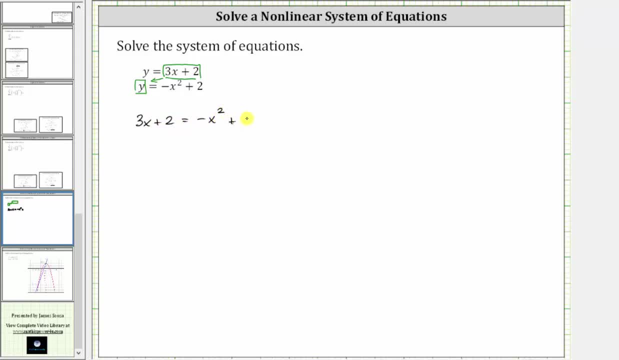 equals negative x squared plus two. Notice how we have a degree two equation or a quadratic equation. So let's set the equation equal to zero and see if we can solve by factoring. We normally prefer to have the x squared term be positive and therefore we will set the right side equal to zero. 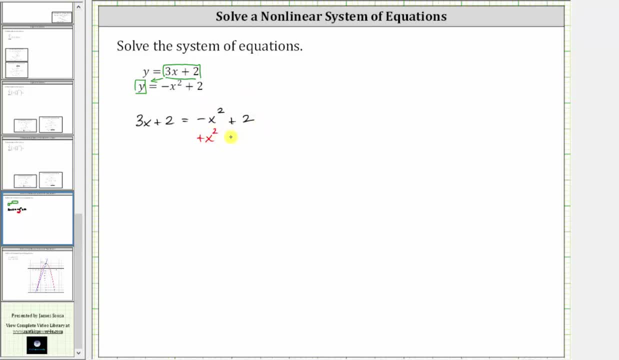 by adding x squared to both sides, as well as subtracting two. And now simplifying: on the left, we have x squared plus three, x, and then two minus two is zero. So on the left, we have x squared plus three x equals on the right side. 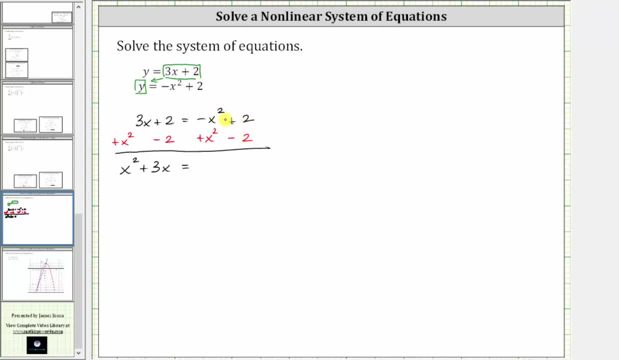 negative: x squared plus x squared is zero, and two minus two is zero, which is the reason why we added x squared to both sides as well as subtracted two on both sides. So the right side is now equal to zero. And now let's factor the left side. 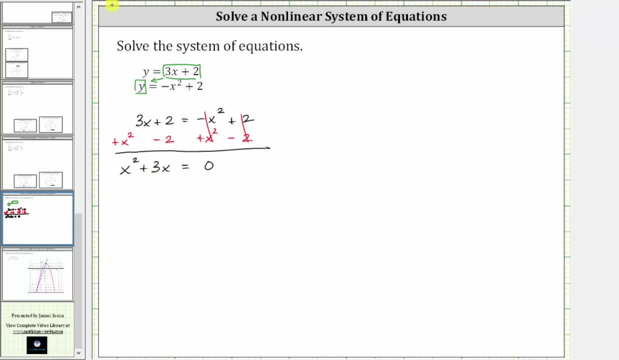 Remember: the first step in factoring is to factor out the greatest common factor. The greatest common factor of x squared plus three, x is x. If we factor out x, we're left with the quantity x plus three. So now we have x times the quantity x plus three equals zero. 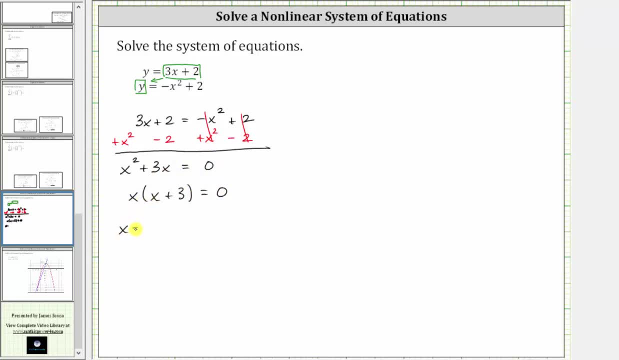 The product on the left is equal to zero when x equals zero, or the factor of x plus three is equal to zero. So one solution to the equation is x equals zero. And now, if we solve this equation, for x we subtract three on both sides. 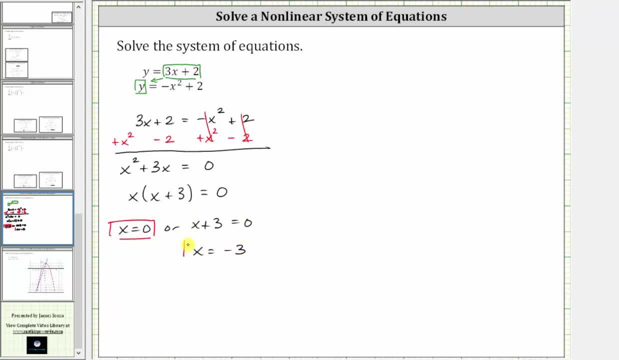 and we have. x equals negative three. But we're not done. Remember, a solution consists of an x and a y value, or an ordered pair in the form of x, comma, y. So we found two possible x values. We now have to find the corresponding y value.